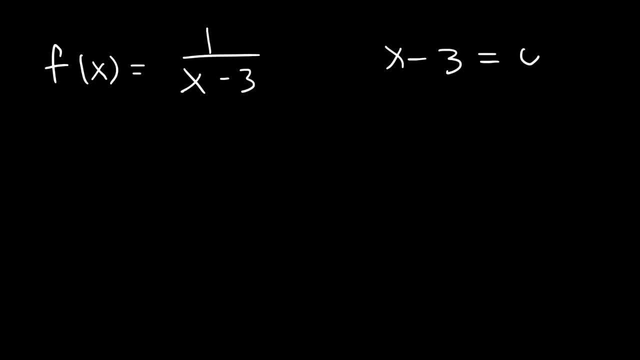 0.. So if you set x minus 3 equal to 0, and if you add 3 to both sides, you'll see that x is equal to 3.. So this is the vertical asymptote, And if you were to graph this function, it would look something like this: So at 3,, we would. 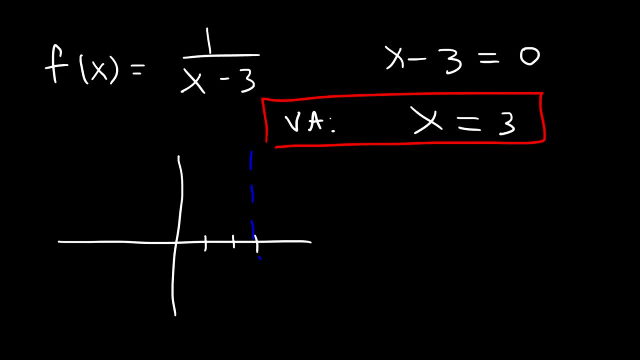 have a vertical asymptote And on the right side the graph is going to be above the x-axis, On the left side, below it. Now let's look at another example. Find the vertical asymptotes in this function: 4 divided by x, squared minus 16.. Now, sometimes you may need to 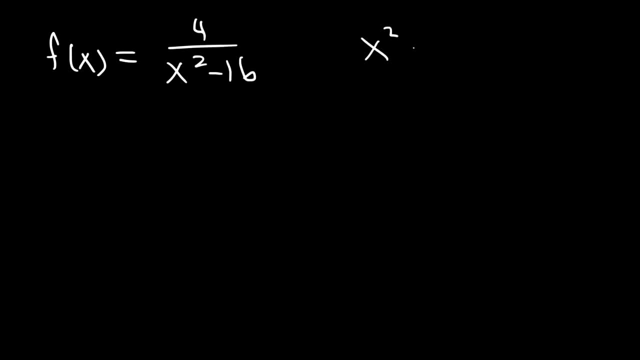 factor the expression. So we could set x squared minus 16 equal to 0.. Now to factor it we could use the difference of squares method. It's going to be x plus 4 times x minus 4.. So in this problem there are two vertical. 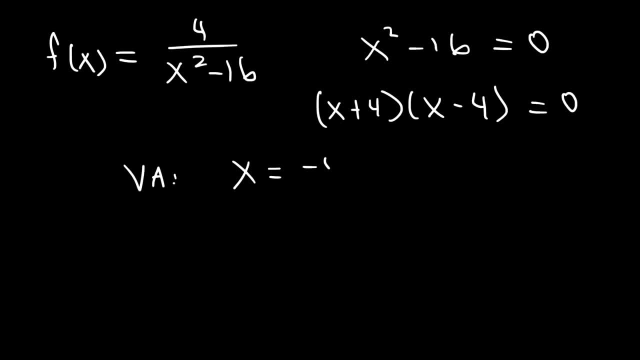 asymptotes. The first one is x squared minus 16.. And the second one is x squared minus 16.. And the first one, x is equal to negative 4.. And the second one, x is equal to positive 4.. Try this one. Let's say, if we have 3x minus 6 divided by x. 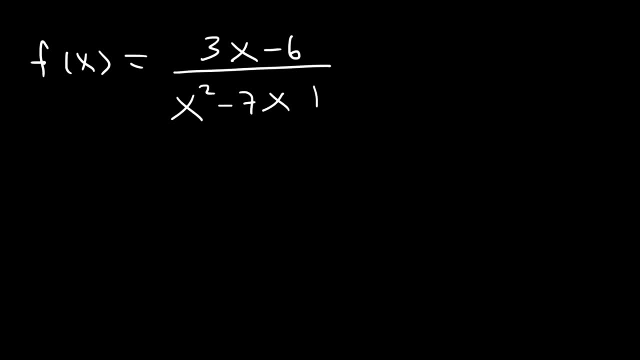 squared minus 7x plus 10.. Go ahead and calculate, or rather find the vertical asymptote. Now, in this problem, you want to factor everything, Including the numerator, So to factor 3x minus 6,. all we could do is take out. 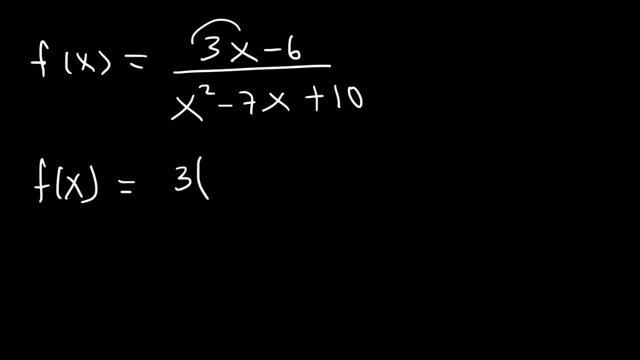 the GCF, the greatest common factor, which is 3.. 3x divided by 3 is x and negative. 6 divided by 3 is negative 2.. Now how can we factor this trinomial If the leading coefficient is 1,? here's what you need to do: Find two numbers. 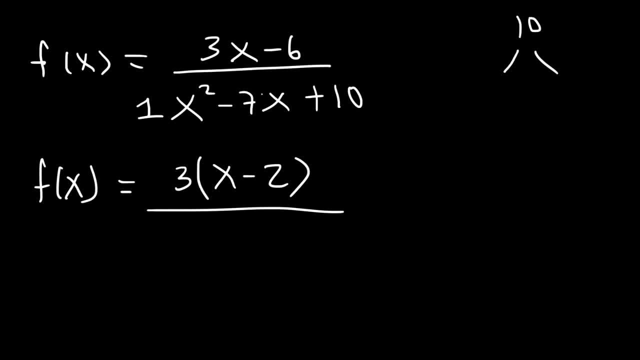 that multiply to 10, but add to the middle one. So if the leading coefficient is the middle term, the middle coefficient negative 7.. So we know 2 times 5 is 10.. And negative, 2 times negative 5 is also positive 10.. But these two add up to negative 7.. 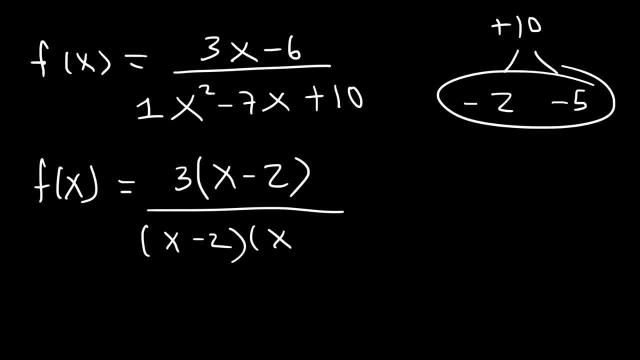 So to factor, it's going to be x minus 2 times x minus 5.. Now notice that we cancel x minus 2.. x equals 2 is a whole, not a vertical asymptote. So what we have remaining is 3 over x minus 5.. 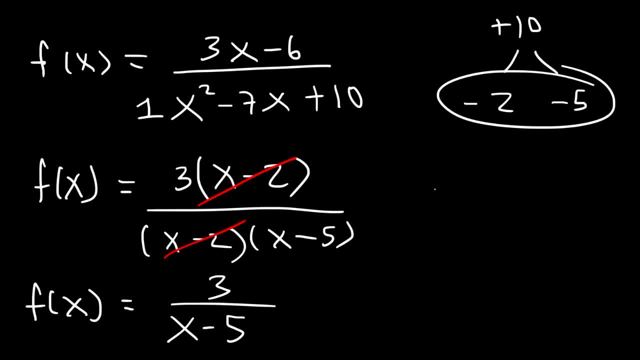 Now there's no way in which we can cancel the x minus 5, so that's what we're going to set equal to 0.. So the vertical asymptote is: x is equal to 5.. Now let's look at another problem. 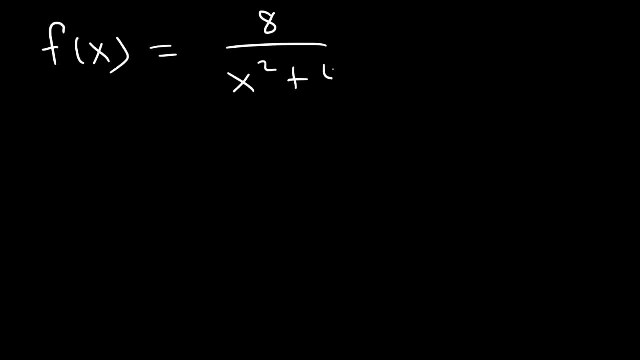 8 divided by x squared plus 4.. Now we can't factor this expression using real numbers, and there's nothing to cancel, so all we could do is set the denominator equal to 0.. Now, if we subtract both sides by 4,, 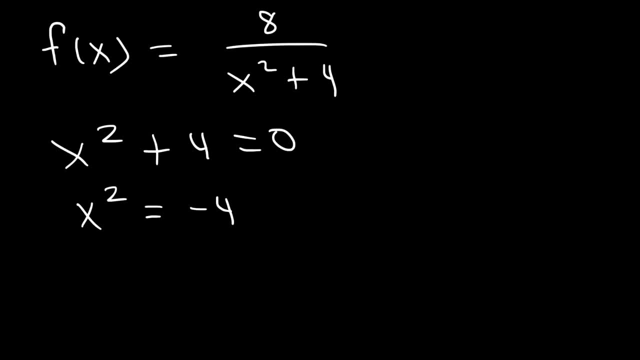 x squared will equal negative 4.. And if we take the square root of both sides, x is going to be plus or minus the square root of negative 4, which is the square root of 4 times the square root of negative 1.. 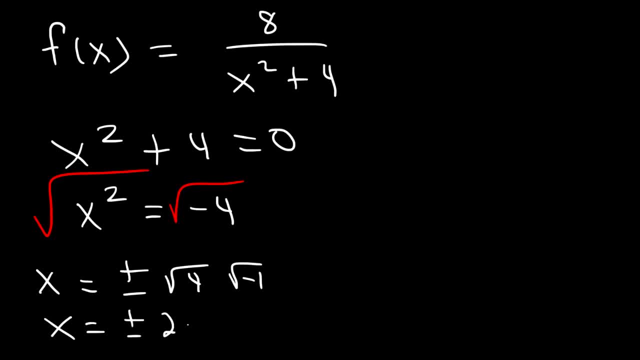 The square root of 4 is 2.. The square root of negative 1 is i. Now, these are imaginary numbers, not real numbers. So therefore we can't have an imaginary vertical asymptote. If you graph it, you won't see a vertical asymptote. 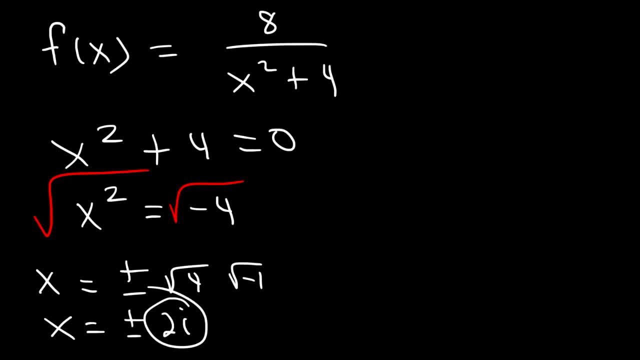 So if you get the situation where x, squared, is equal to a negative number, or any even exponent is equal to a negative number, you're not going to get a vertical asymptote for this problem, So there's none. So if you get an imaginary solution, there's no vertical asymptotes. 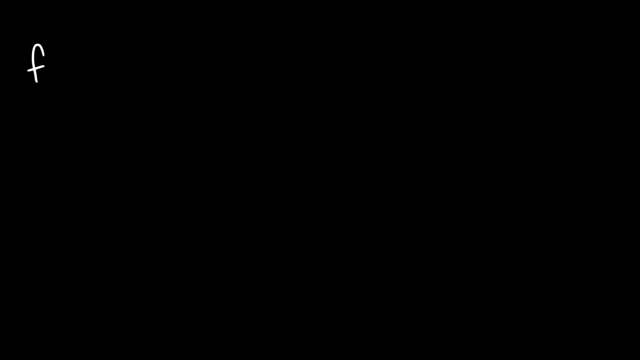 Now let's look at one final example. This one might be- This might be harder than the previous ones, but you can try it as well. Let's say: f of x is equal to 10x squared minus 5x minus 15. 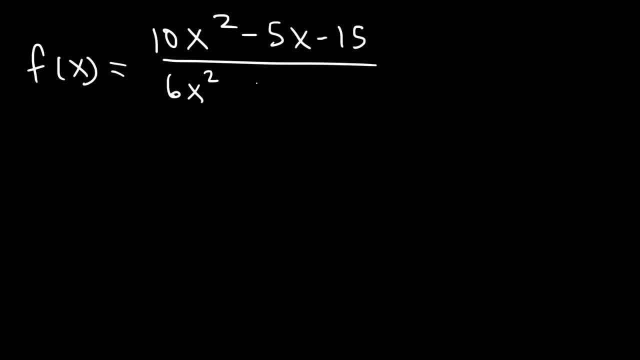 divided by 6x squared minus 17x plus 12.. Find the vertical asymptotes. So let's start by factoring the numerator. So I'm just going to write it right here: 10x squared minus 5x minus 15.. 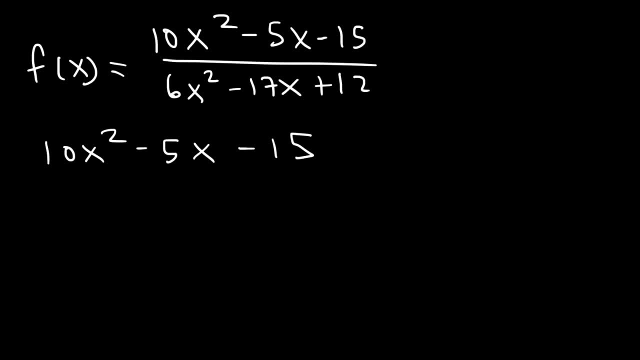 So how should we factor this? How can we begin? The first thing you should do, if possible, is to remove the GCF. The greatest common factor is 5.. So 10x squared divided by 5 is 2x squared. 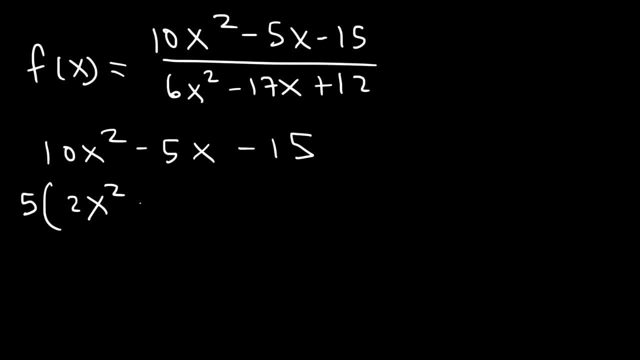 Negative 5x divided by 5 is negative 1x. or simply negative x And negative 15 divided by 5. is negative 3.. So now we need to factor this expression. If you want to factor a trinomial where the leading coefficient is not 1,. 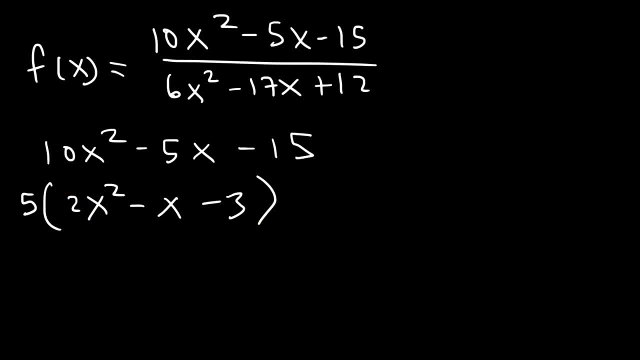 multiply the leading coefficient by the constant term. So 2 times negative 3 is negative 6.. Now we need to find two numbers that multiply to negative 6, but add to the middle coefficient negative 1.. So that's going to be the same numbers, 2 and negative 3.. 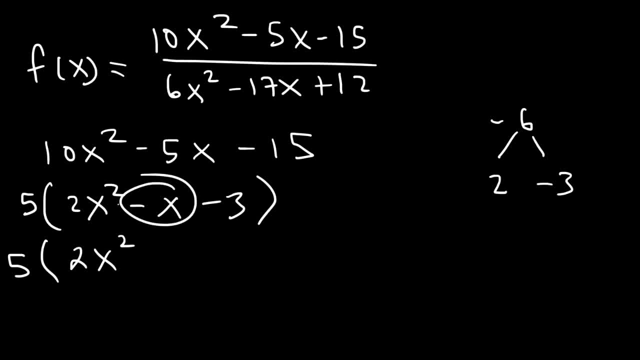 So I'm going to replace the middle term negative x with positive 2x and negative 3x, Because those two they add up to negative x. And then what you need to do at this point is you need to factor by grouping. 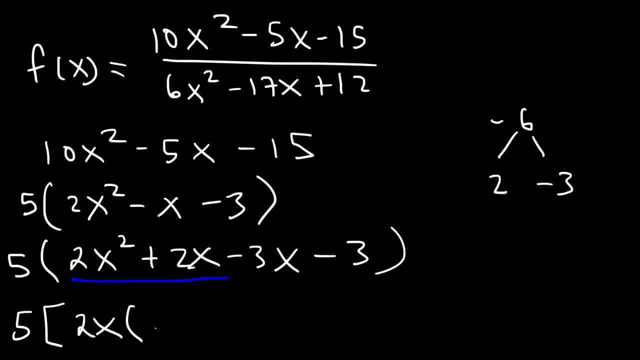 So in the first two terms I can take out a 2x- 2x squared divided by 2x is x and 2x divided by 2x is 1.. And the last two terms take out a negative 3.. 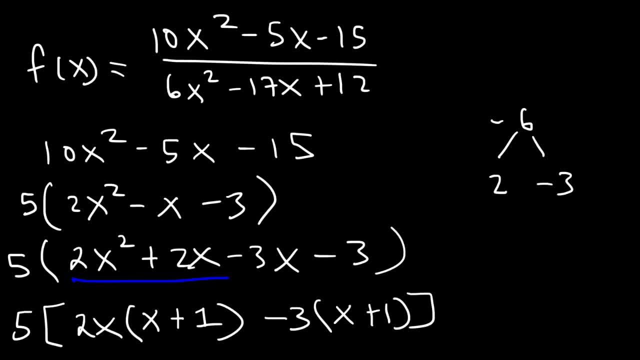 So we'll be left with x plus 1.. Now, if these two terms are the same, then you know you're on the right track. So now we need to factor out x plus 1.. And so what we have left over is 2x minus 3.. 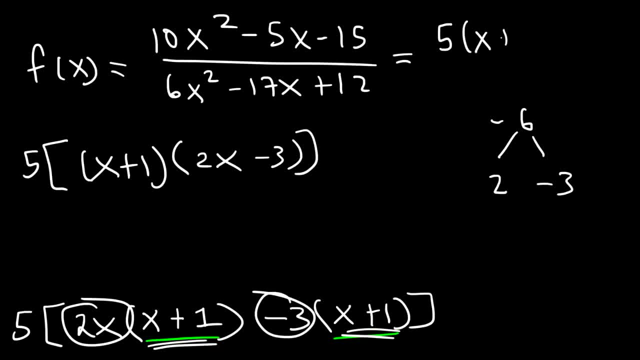 So the numerator is 5 times x plus 1.. Times 2x minus 3.. Now we need to do the same thing for the denominator. How can we factor the denominator? What can we do? What we need to do is multiply the leading coefficient by the constant term. 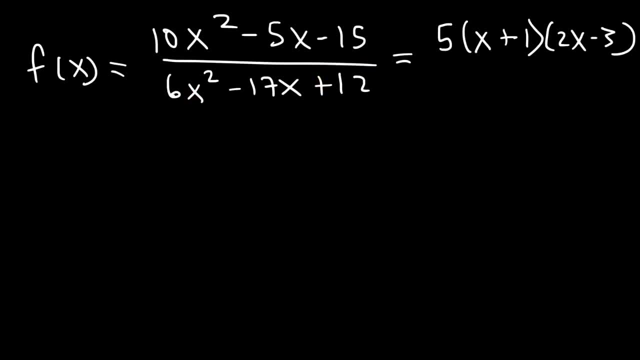 There's no GCF that we can factor, so we're not going to worry about that. We can't take out a 6 from negative 17.. Now 6 times 12,, that's 72. Now we need to find two numbers that multiply to 72, but add up to negative 17.. 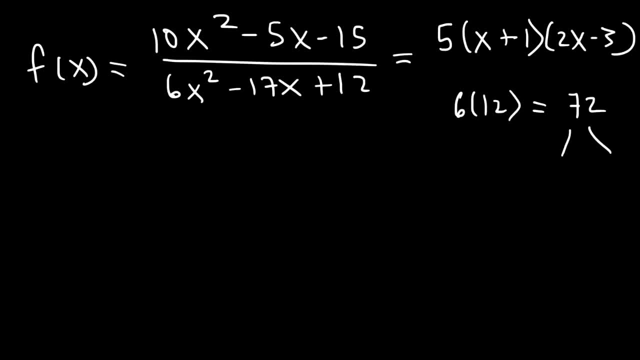 So we need two negative numbers, But for now I'm just going to use positive numbers and then I can change the sign later. So 2 goes into 72 36 times, 3 goes into it 24 times, And then you can just go in order. 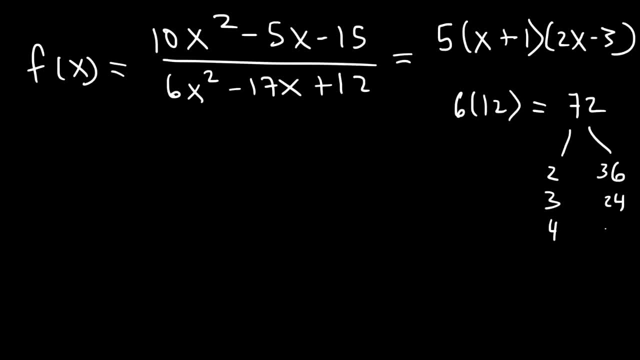 Until you get two numbers that add up to 17.. 4 goes into it. 18 times 72, divided by 4, is 18.. If you divide it by 6, you'll get 12.. Now, factors of 6 are 2 and 3.. 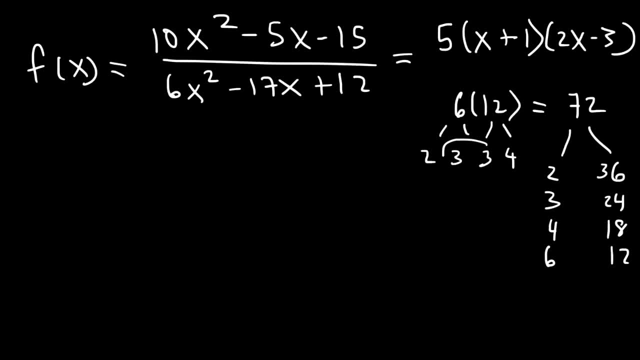 Factors of 12 are 3 and 4. So notice that we can get a 9 out of it. 3 times 3 is 9.. So 72 divided by 9 is 8.. And 9 plus 8 adds up to 17.. 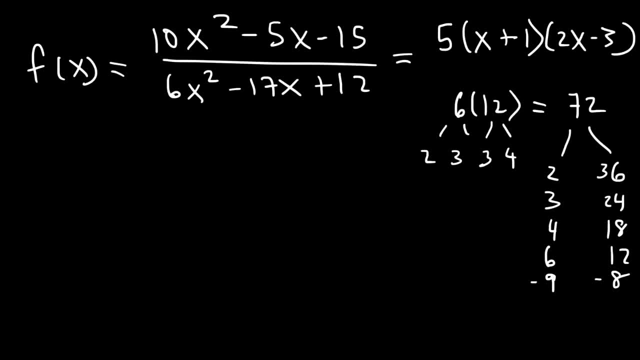 So we're going to use negative 9 and negative 8.. If you have large numbers like 72, it might be good to make a list. If you make a systematic list and just go in order, you will find it eventually if it's factorable. 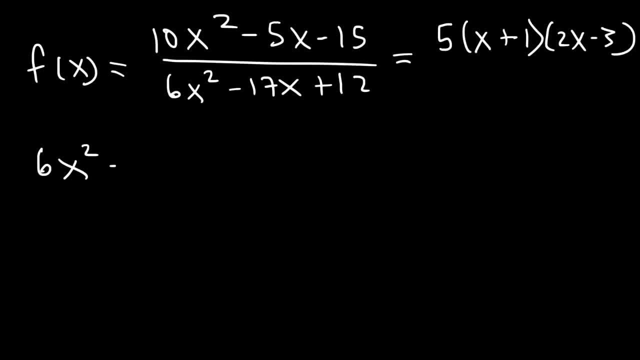 So now I'm going to replace negative 17x with negative 9x, Actually with negative 8x minus 9x. The order in which you place it doesn't matter, But 6 and 8 are even numbers, so I'm going to put them together. 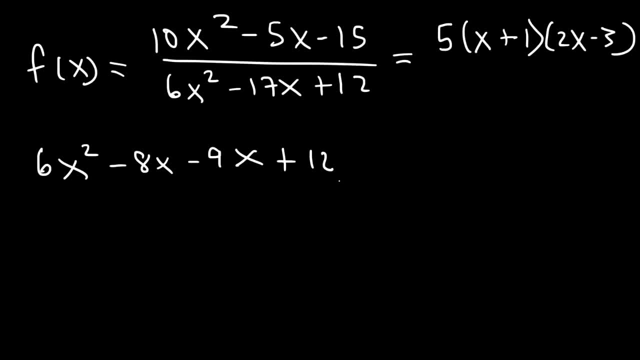 And 9 and 12, I guess you could take out a 3 from both of them. Now let's factor by grouping In the first two terms, we could take out a 2x. 6x squared divided by 2x is 3x. 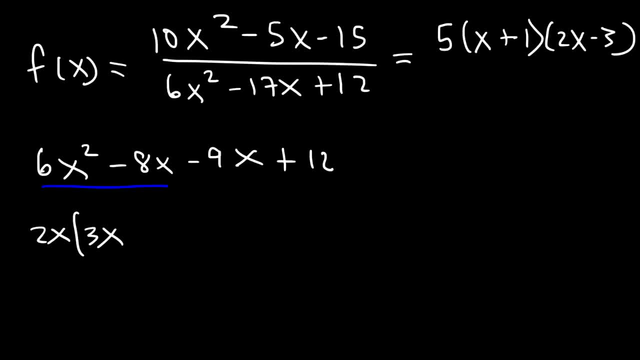 And negative: 8x divided by 2x, that's negative 4.. In the last two terms we could take out A negative 3.. Negative 9x divided by negative: 3 is positive. 3x 12 divided by negative: 3 is negative 4..